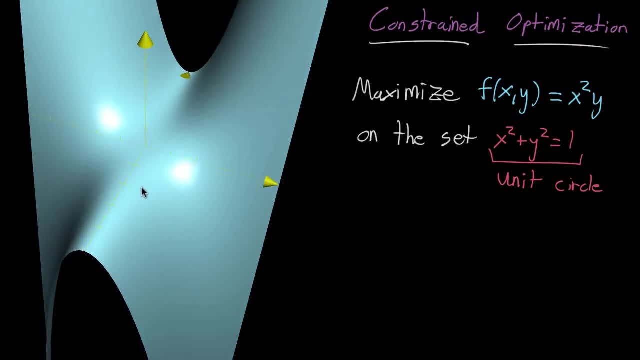 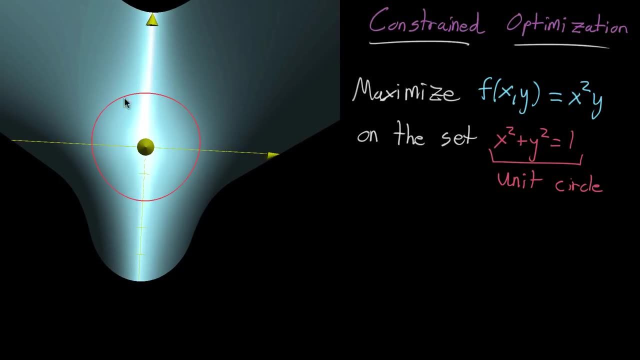 And now this constraint, x squared plus y squared, is basically just a subset of the xy plane. So if we look at it head on here and we look at the xy plane, this circle represents all of the points xy, such that this holds, And what I've actually drawn here isn't the circle on the xy plane. 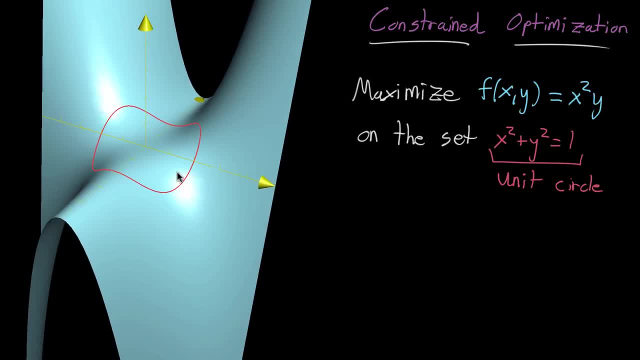 but I've projected it up onto the graph. So this is showing you basically the values where this constraint holds and also what they look like when graphed. So a way you can think about a problem like this is that you're looking on this circle, this kind of projected circle onto the graph. 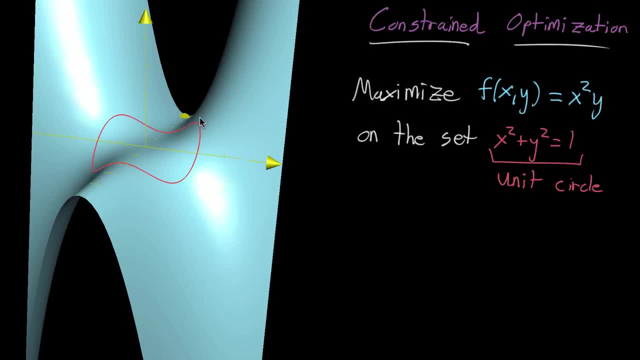 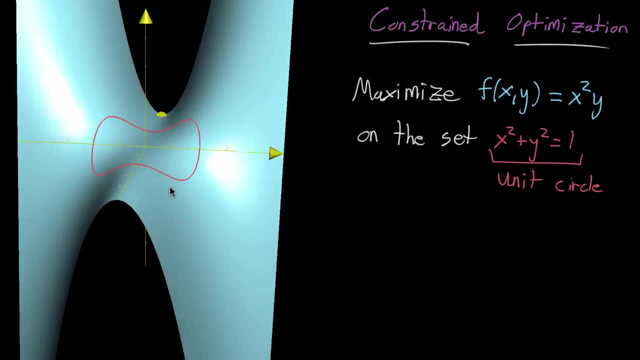 and looking for the highest points And you might notice kind of here there's sort of a peak on that wiggly circle, and over here there's another one, And then the low points would be around that point and around over here. Now, this is good and I think this is a nice way to sort of wrap your head around. 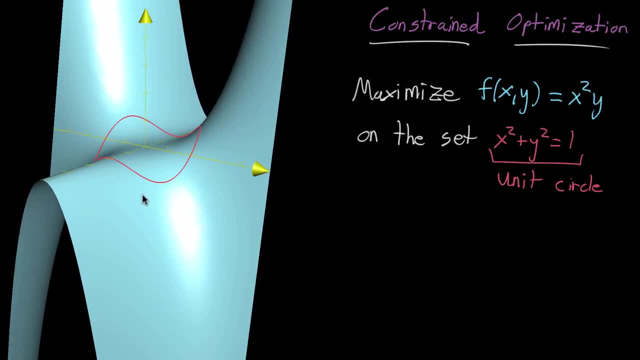 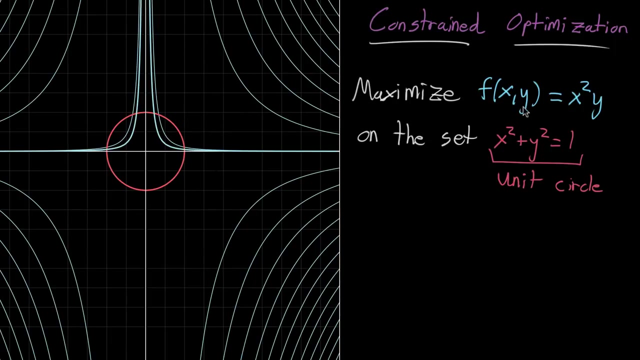 what this problem is asking. But there's actually a better way to visualize it in terms of finding the actual solution, And that's to look only in the xy plane, rather than trying to graph things and just limit our perspective to the input space. So what I have here are the contour lines, for f of xy equals x squared plus y squared. 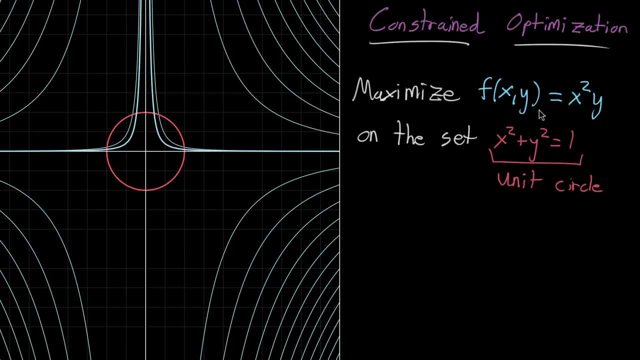 And if you're unfamiliar with contour lines or contour map, I have a video on that you can go back and take a look. It's going to be pretty crucial for the next couple videos to have a feel for that, But basically each one of these lines represents a certain constant value for f. 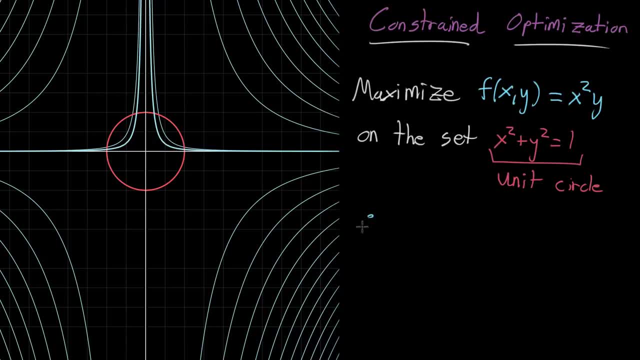 So, for example, one of them might represent all of the values of x and y, where f of xy is equal to 2.. So if you looked at all the values of x and y where this is true, you'd find yourself on one of these lines. 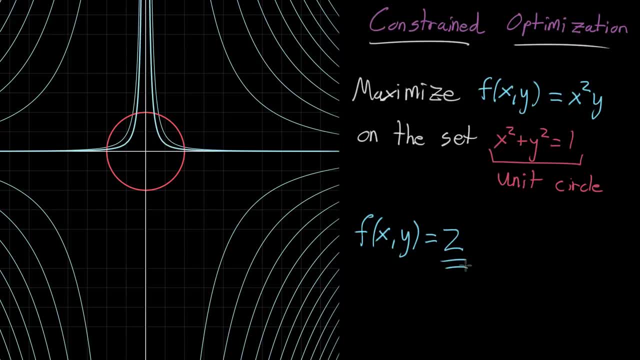 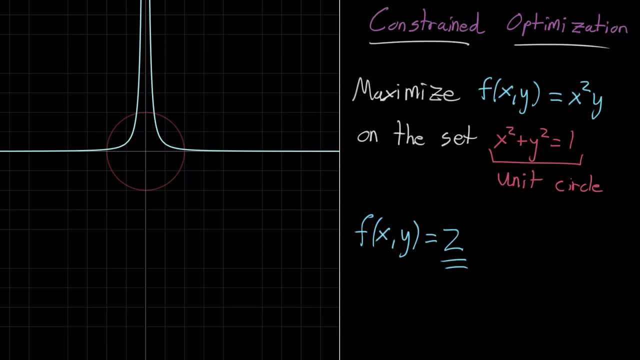 And each line represents a different possible value for what this constant here actually is. So what I'm going to do here is I'm actually going to just zoom in on one particular contour line. So this here is something that I'm going to vary, where I'm going to be able to change what the constant we're setting f equal to is. 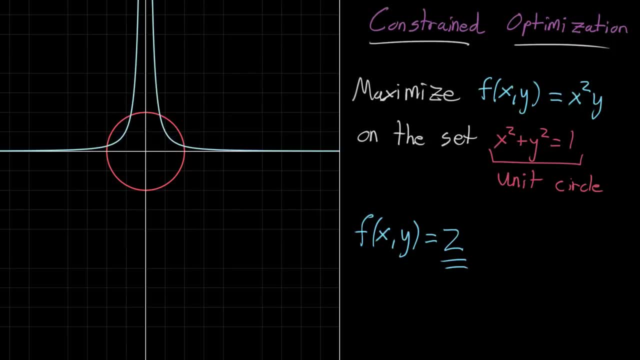 and look at how the contour line changes as a result. So, for example, if I put it around here-ish, what you're looking at is the contour line for f of xy equals 0.1.. So all of the values on these two blue lines here. 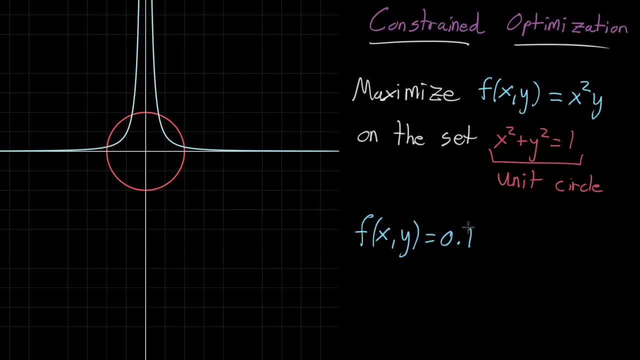 will tell you what values of x and y satisfy 0.1.. But on the other hand, I could also shift this guy up and maybe I'll shift it up. I'm going to set it to where that constant is actually equal to 1.. 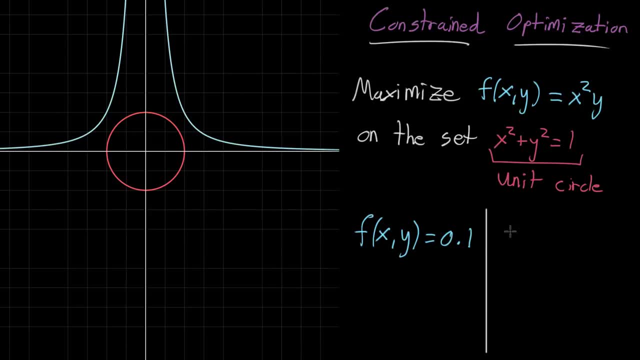 So that would be kind of an alternative. I'll just kind of separate over here. That would be the line where f of xy is set equal to 1 itself, And the main thing I want to highlight here is that at some values like 0.1. 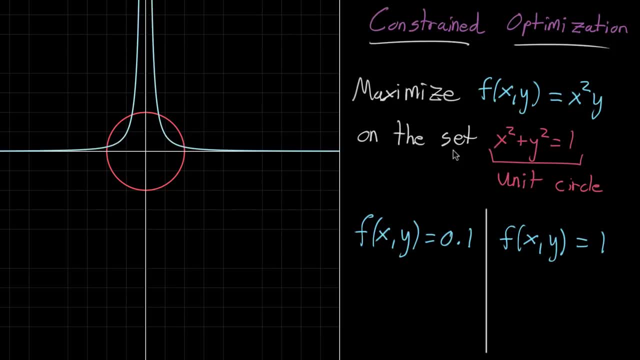 this contour line intersects with the circle, It intersects with our constraint, And let's just think about what that means. If there's a point x and y on that intersection there, that basically gives us a pair of numbers, x and y, such that this is true, that fact that f of xy equals 0.1. 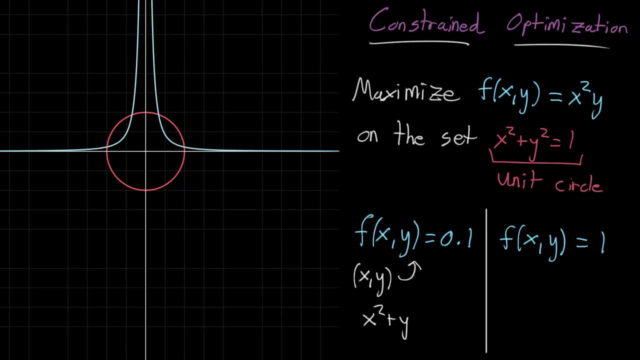 and also that x squared plus y squared equals 1.. So it means this is something that actually exists and is possible, And in fact we can see that there's four different pairs of numbers where that's true, where they intersect here, where they intersect over here. 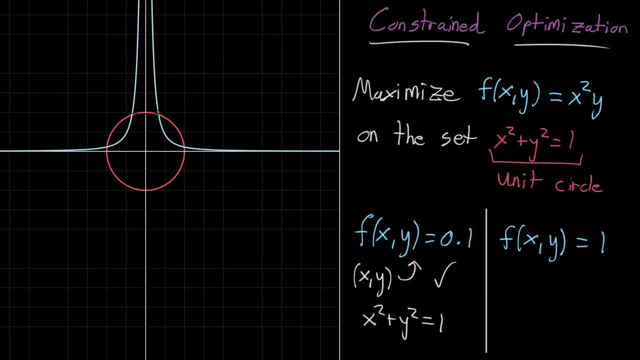 and then the other two kind of symmetrically on that side. But on the other hand, if we look at this other world where we shift up to the line f of xy equals 1, this never intersects with the constraint, So what that means is xy. 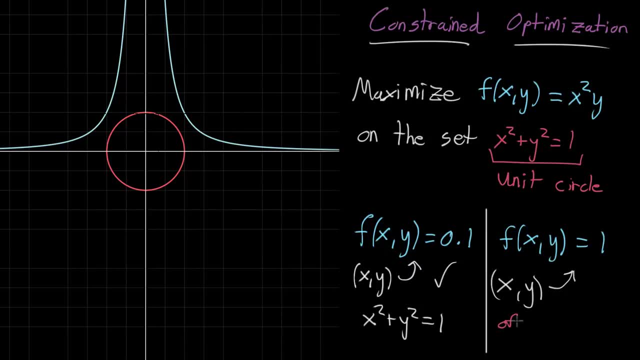 the pairs of numbers that satisfy this guy are off the constraint. They're off of that circle. x squared plus y squared equals 1.. So what that tells us, as we try to maximize this function subject to this constraint, is that we can never get as high as 1.. 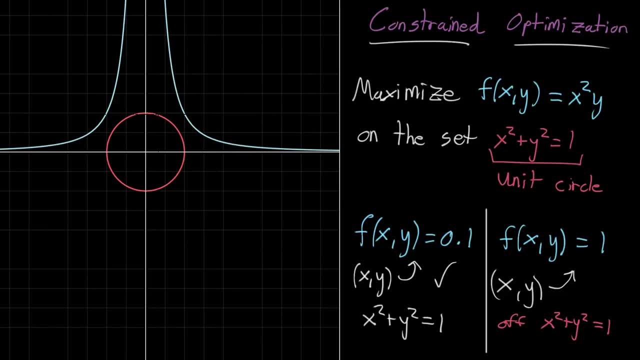 0.1 would be achievable. And in fact, if we kind of go back to that and we look at 0.1, if I upped that value and changed it to the line where, instead, what you're looking at is 0.2,.